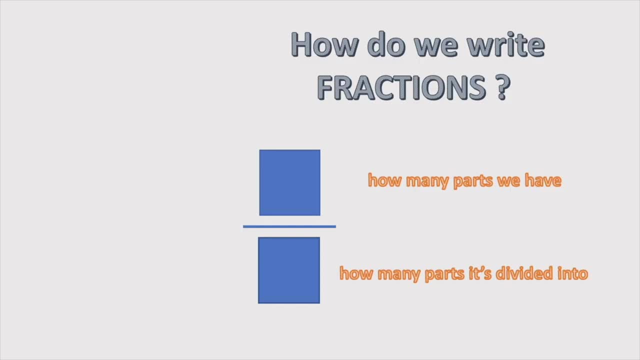 What happens if one part is taken out of the whole? Well, the circle is still divided into eight equal parts. Therefore, the bottom number will still be eight, While the top number will be seven, because we only have seven left. Our fraction is seven eighths. 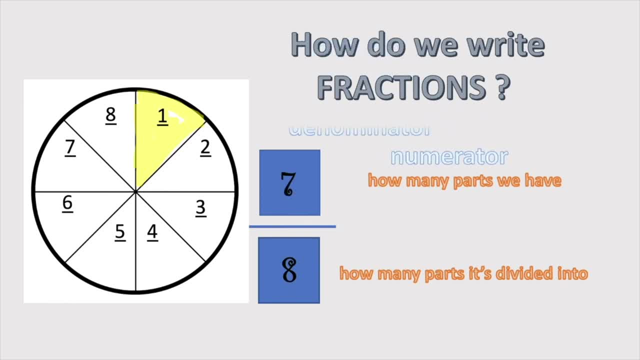 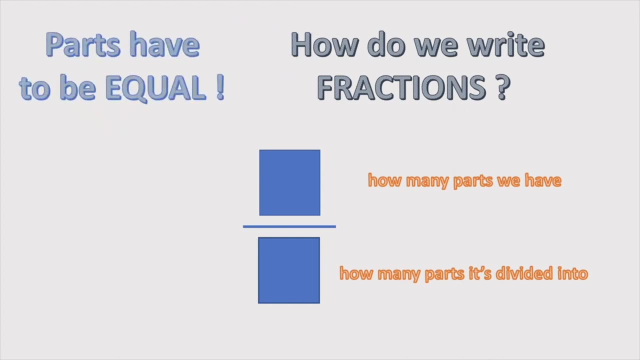 The top number is called numerator, While the bottom number is called denominator. Now remember, the part that you divide the whole into should be equal. Now let's have this example before we checked on Emily's baking: The shaded part represents the part that is taken away. 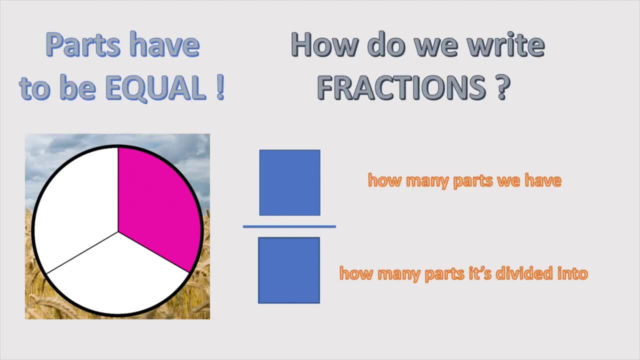 How many parts is the whole divided into? You're correct: Three. Now how many parts is left? Good job, Two thirds. Using the same example, can our answer be a different fraction? Yes, it can. It depends on the question. 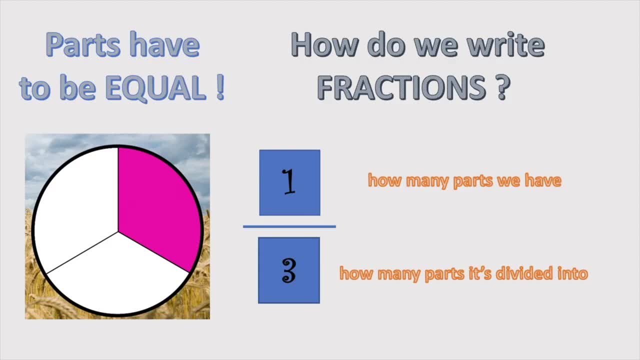 If the question asks for what part is shaded pink, our answer is going to be one third. If the question asks for what fraction part is taken or given away, then our answer will be one third. Okay, let's go ahead and check on Emily's baking. 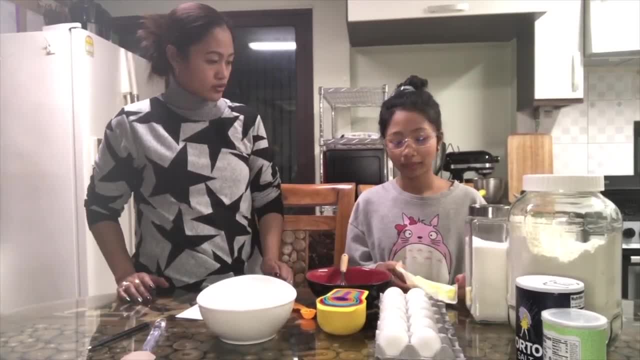 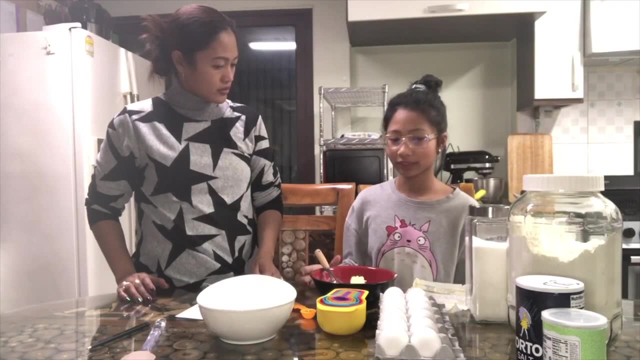 Okay, so let's start baking. What's the first thing that you do? Butter, Butter, Okay, butter. Then, after the butter, what's next? Three fourths cup of sugar. Did you hear that? Three fourths cup of sugar? 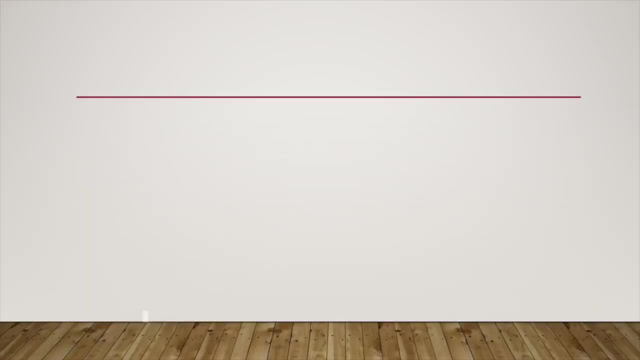 How would Emily measure the correct amount of sugar she needs? Let's have some illustrations. Emily is using a measuring cup to measure her dry ingredients. One cup will represent our whole and she needs three fourths cups of sugar. Use your knowledge of fractions to know how to measure the sugar Emily needs. 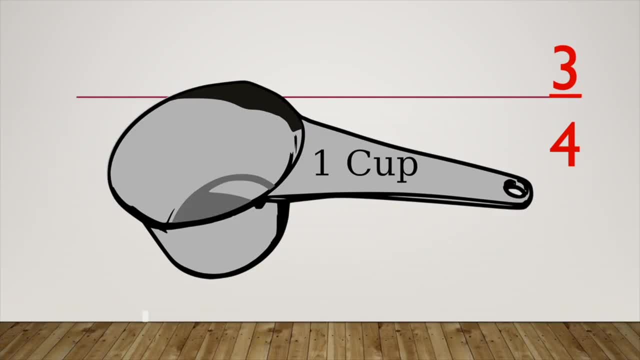 We know that the denominator tells us how many parts we divide the whole into. In this case we divide it into four equal parts. Each part is one part out of the four total parts. or we can say one fourth- Emily needs three from those four total parts. 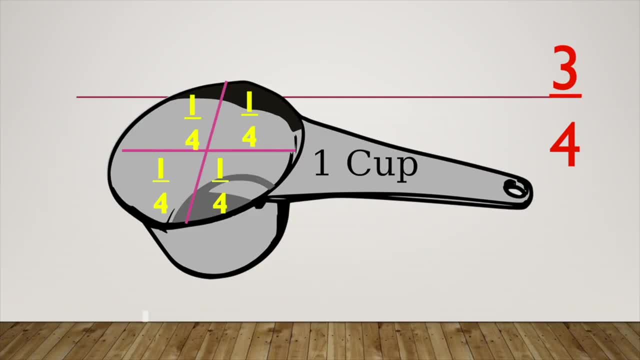 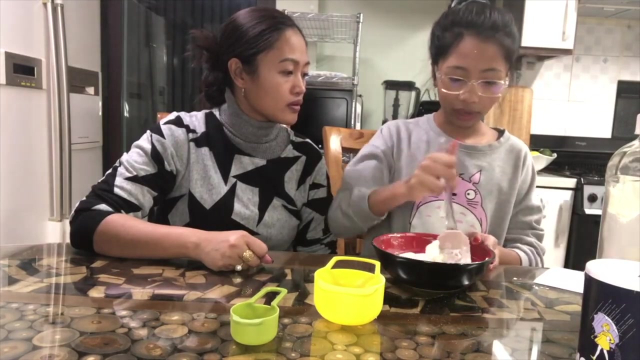 She needs three fourths. Emily also has one fourth measuring cup, So she will use the one fourth measuring cup three times. for her to measure three fourths sugar that she needs, We need one and three fourths cup of flour. Okay, Now we need one and three fourths cup of flour. 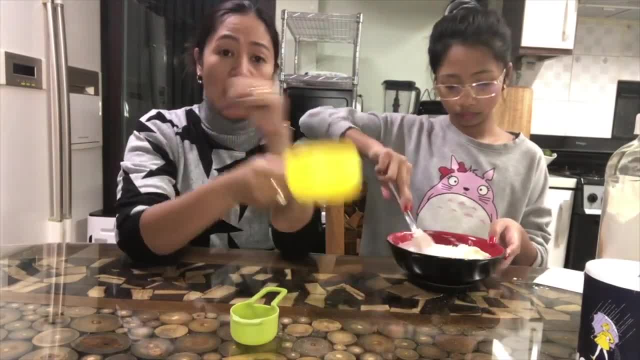 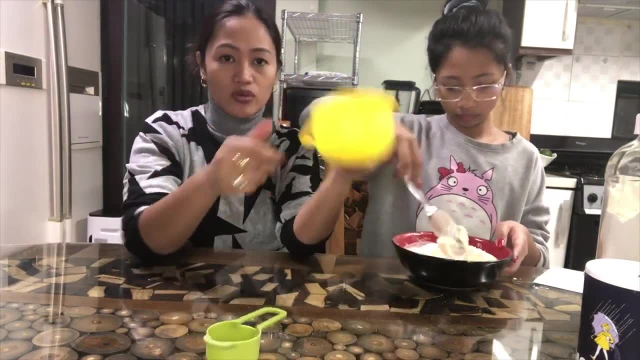 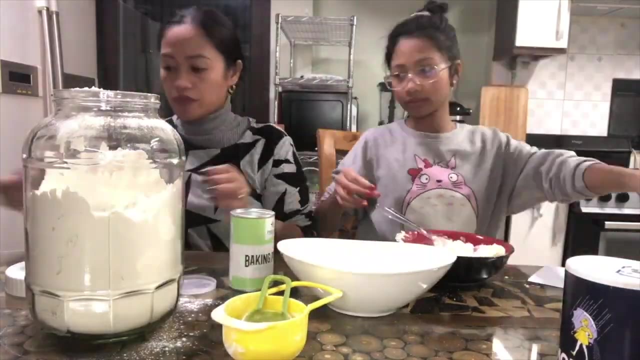 So that means we need one whole and three fourth cups. Remember, this is one fourth, So to make three fourths we need three of this. right, So we need one cup plus three of this Flour. Okay, so let's have this. 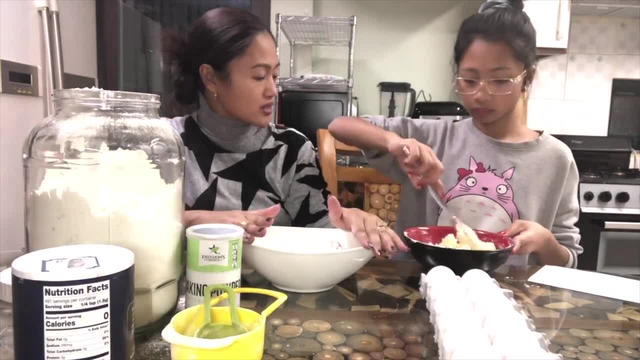 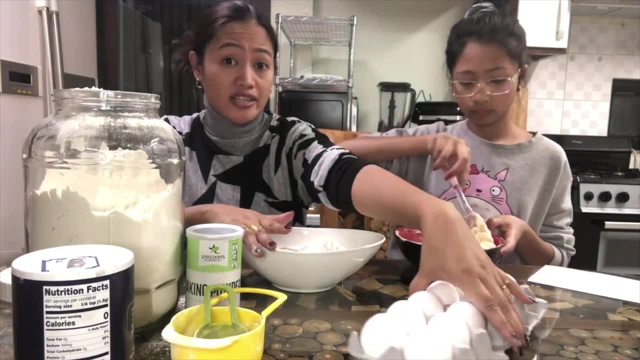 Okay. so after the flour and the baking powder, what's next? Now we need one egg to add to this mixture. Okay, one egg Now. when we buy eggs, usually they come in dozen. Okay, so one dozen is equal to twelve pieces. 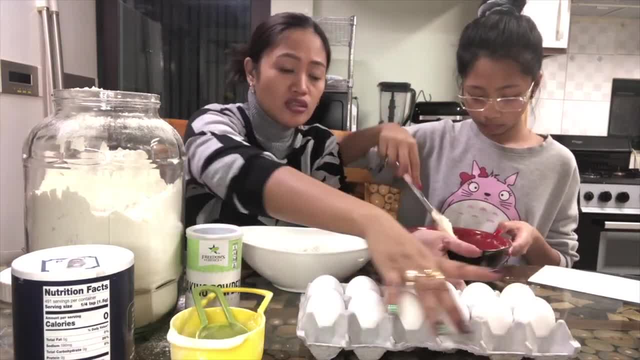 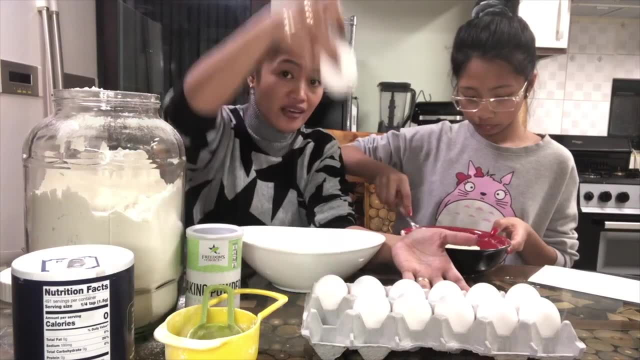 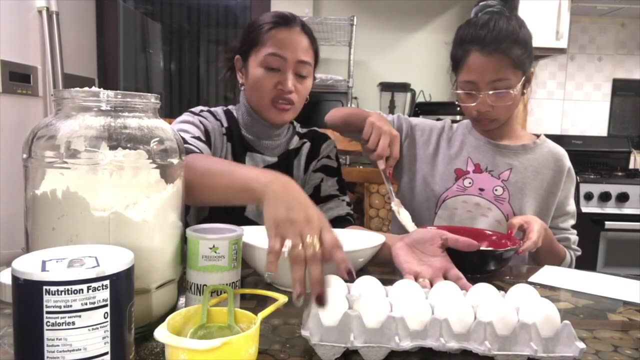 Now we can relate fraction to this again. So this twelve eggs is considered one whole And each part of this whole, each piece of egg, is considered a fraction, So one out of the twelve pieces. Okay, so this is like our one whole. 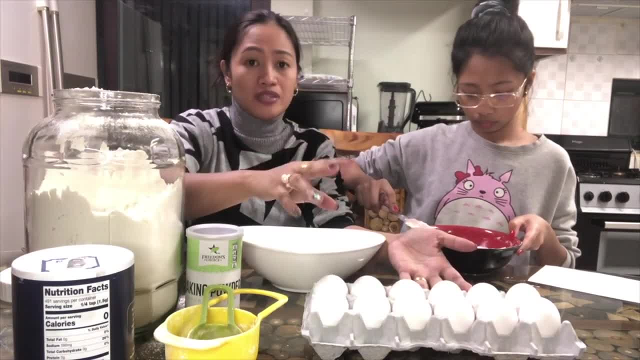 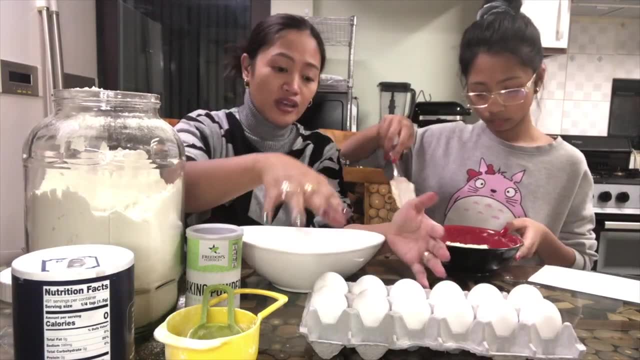 And we split it into twelve pieces, which is represented by our twelve eggs. So one egg is one part of those twelve pieces. So get four eggs. that's going to be four of the twelve, The twelve total. so it's going to be four twelves. 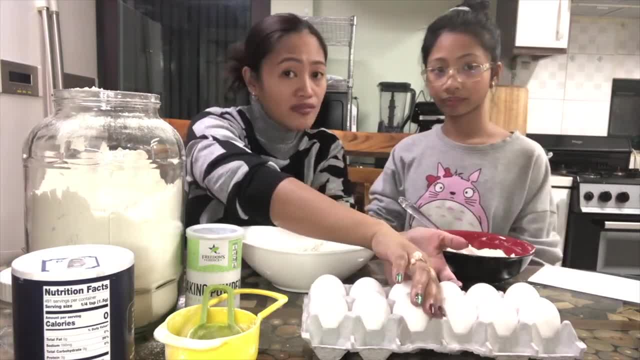 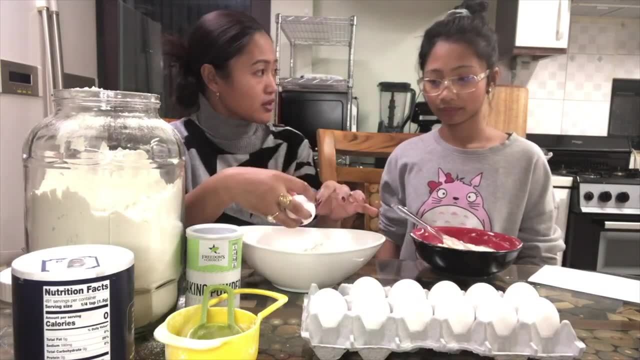 If I get six eggs, that's going to be six of the twelve, so that's going to be six, twelves, Okay, so how many eggs do we need? One, Just one. So will I just break it in the middle.